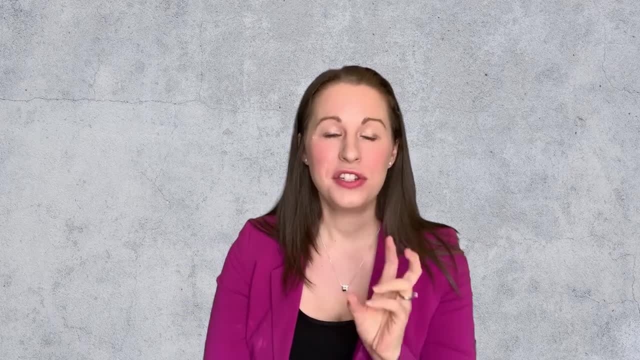 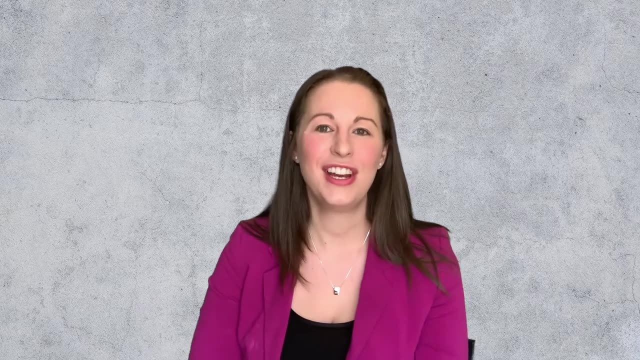 got to consider is: what name are you going to use Now? don't worry, If you pick a name now, it's not the end of the world. You can change it in the future if, for whatever reason, you're not really feeling it at a future date. It is important, but it isn't at the same time, So I'd just say: 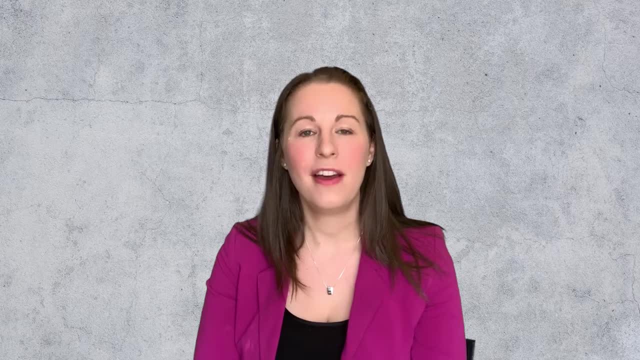 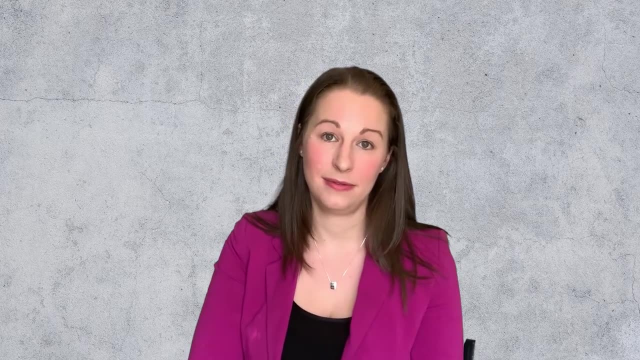 don't hold off on doing things just because you've got a name. Figure one out, and if you figure a better one out in the future, you can. You can change the name later. So the next thing to consider is: who are the shareholders going to? 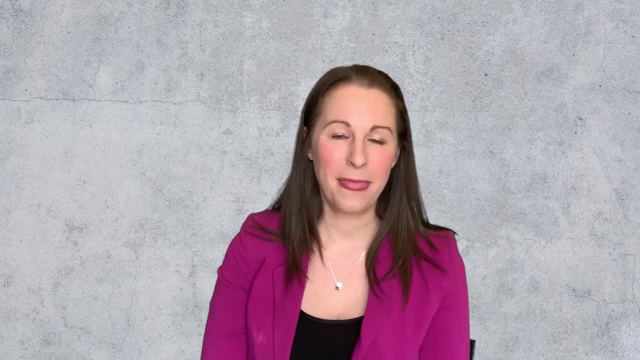 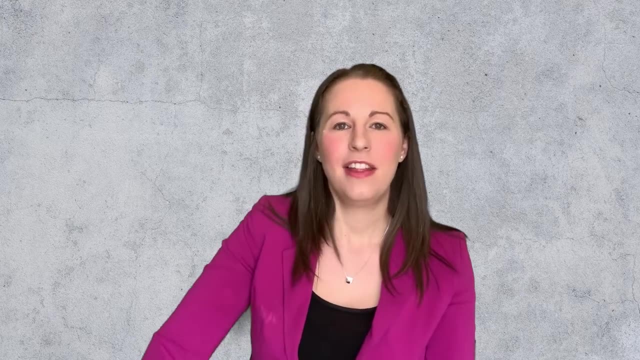 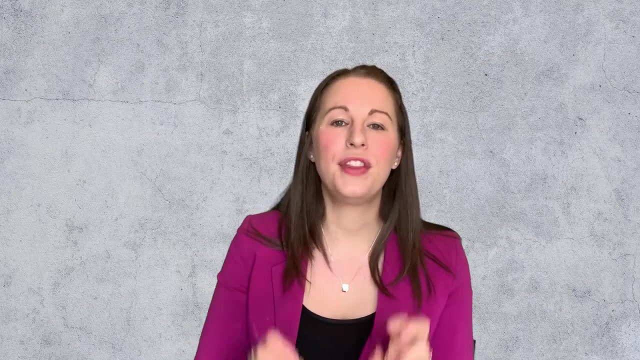 be? Who are the directors going to be? So let's just have a look into them for a second. What are shareholders? So let's think of those big companies out there, the likes of Rolls-Royce, GlaxoSmithKline. There's a lot of shareholders out there. They're all the people that own the. 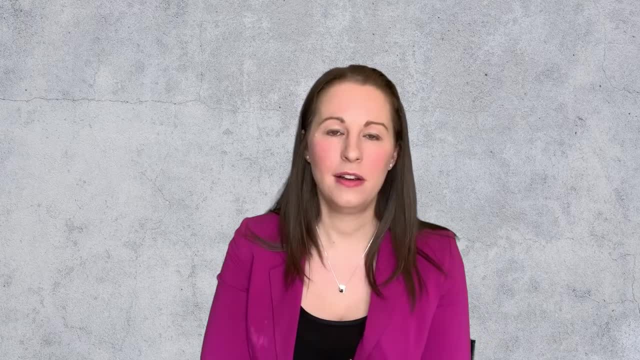 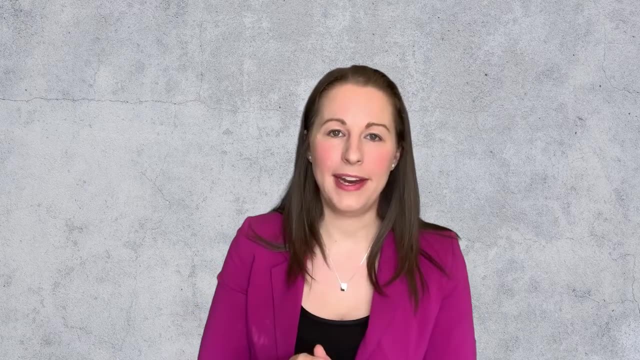 company. So, potentially, you maybe your partner, maybe a business partner, maybe a business partner maybe your children, maybe your grandchildren. They're going to be the owners of the company. So we'll talk about shareholders in a second to figure out what is going to be the right. 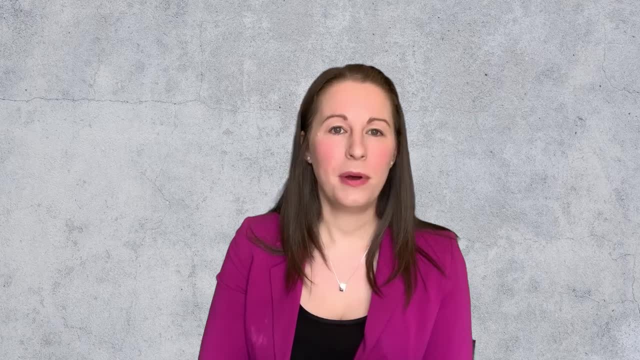 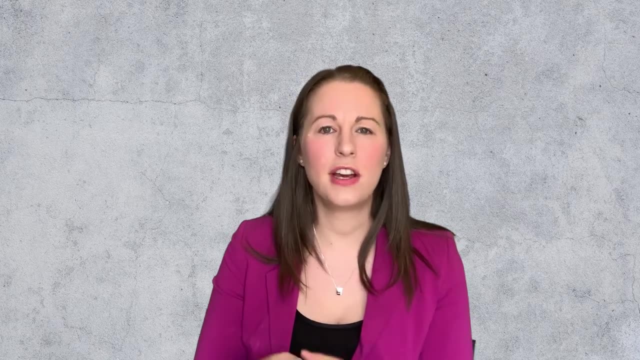 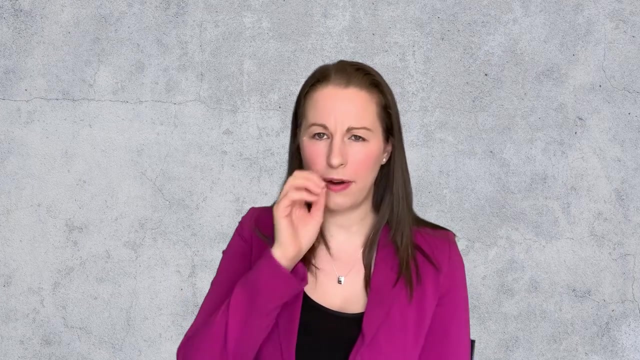 option for you and how you set it up, But they are the ones who own the company. Let's move on to the directors now. The directors: they're the ones that control the company, So they're the ones that make the day-to-day decisions. They're the ones who are going to be the ones on the ground signing off all. 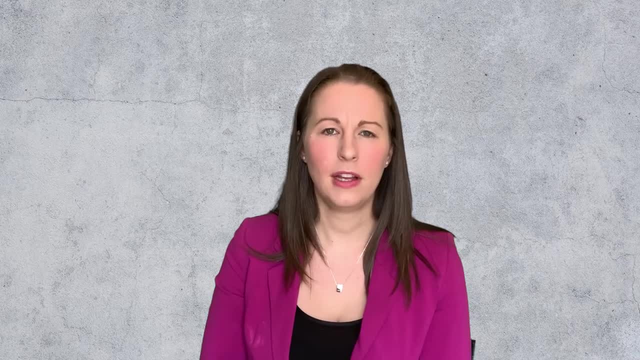 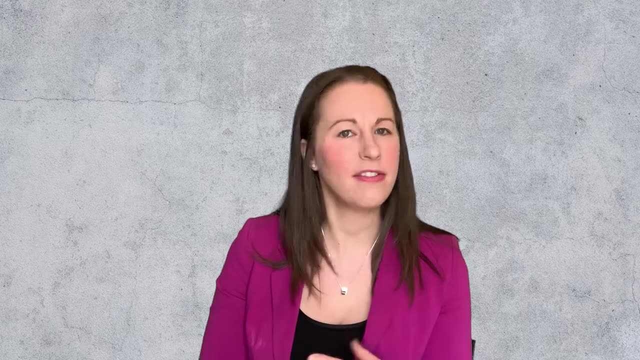 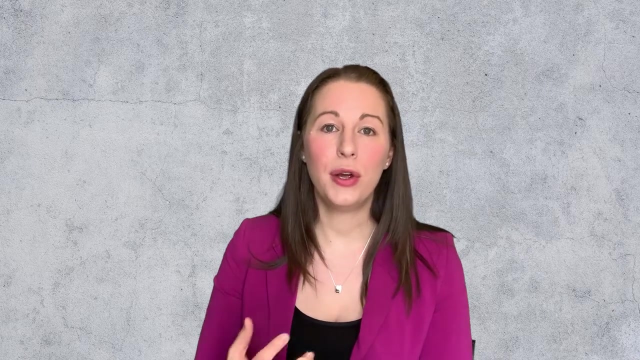 work and dealing with everything. Now you can have as many or as few directors as you want, So you can have one director if that's the right decision, Or if you want to have more than one director, you can. There's no limit. You just need to figure out who is going to be the right person. 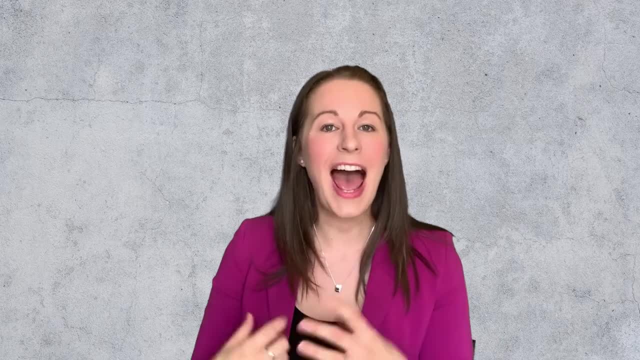 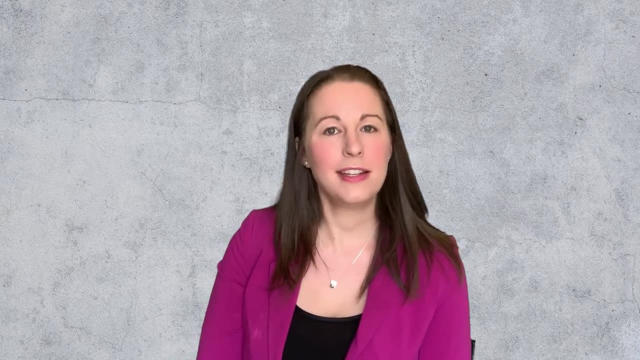 or persons to be the directors of the company and take responsibility In terms of the number of shares that you have in the company. I see a lot of people who are going to be the directors of the company. There are a lot of people who just set it up with one share each. Now I would tend to recommend against that And I would suggest that you have at least 10.. You might even go as far as 20 or 100 shares. Now the reason I say to have 10 or 20 or 100 really comes down to choice in the. future, Because you might set it up with you and your spouse now and have 10 shares each, But in the future you might want to bring more people in, such as children or grandchildren. So if you set it up with 20 shares now, that gives you options for the future. So I would tend to suggest, as a minimum, have 10 shares, but maybe go for 20 or 100. And then that just gives you choice and options in the future For your shares. you may wish to set them up as alphabet shares. Now, alphabet shares are different share classes, So you would have an A class. 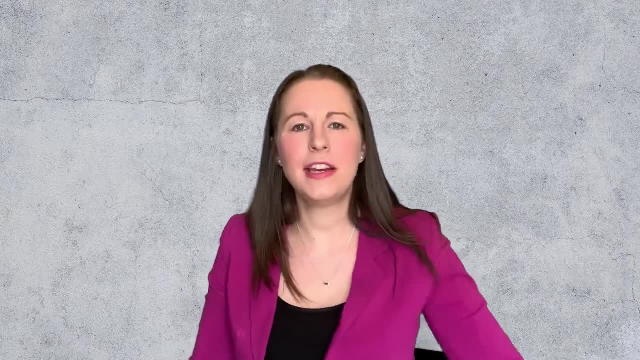 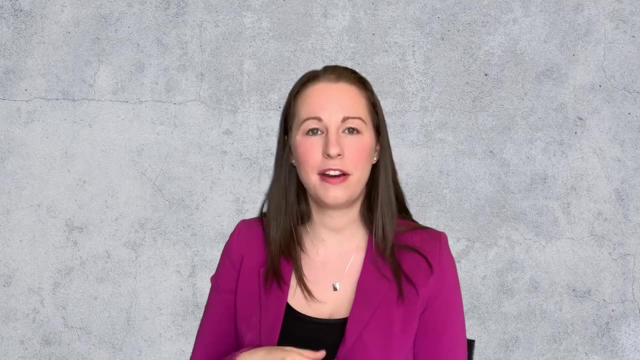 a B class, a C class, And what this means is a different class can have different dividends voted to them. So this works really well in the future as the company starts generating income. So let's say there's 10,000 of income and you 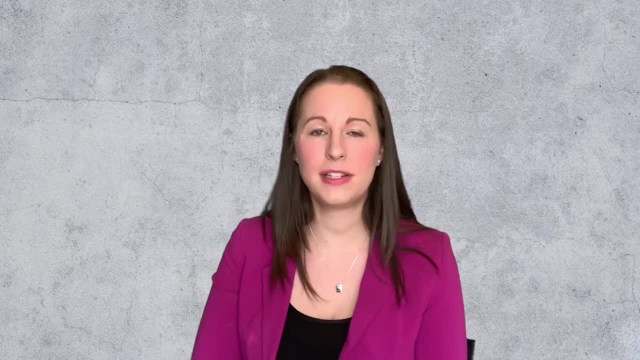 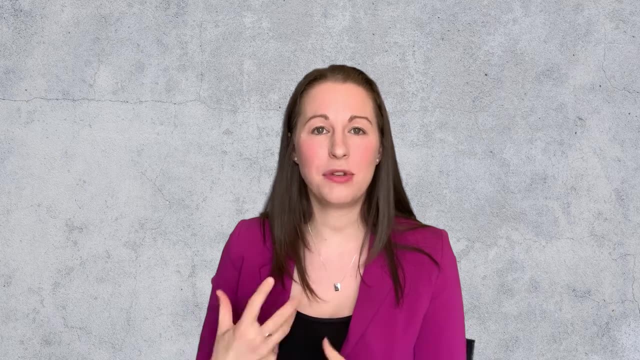 want to give maybe one of your children 1,000 pounds and you want to give another of your children 1,000 pounds, But you personally you want to take 5,000.. Now if you all have the share class, you would all have to have the same dividend, which kind of means you potentially 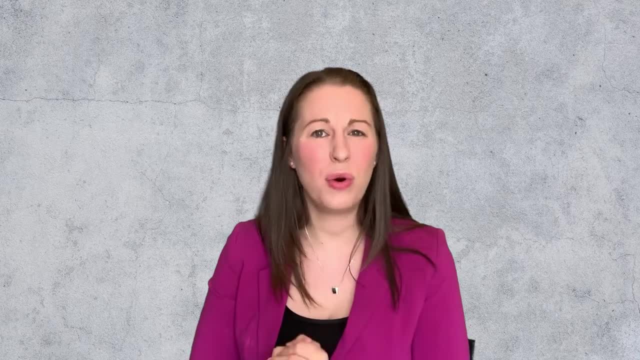 would all have to have 1,000, which would be the same share class. So if you all have the same share class, you would all have to have the same dividend, which kind of means you potentially wouldn't necessarily give you what you're looking to take out, Whereas if you've got A shares and B shares and C shares, you as an A shareholder, could have 5,000.. And then you could have the B and the C shareholder. both have 1,000.. Now this is some great planning opportunities and also great from an inheritance tax point of view as well, which we'll be covering in a separate. 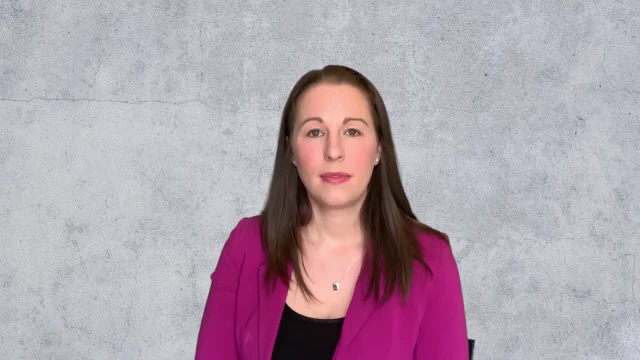 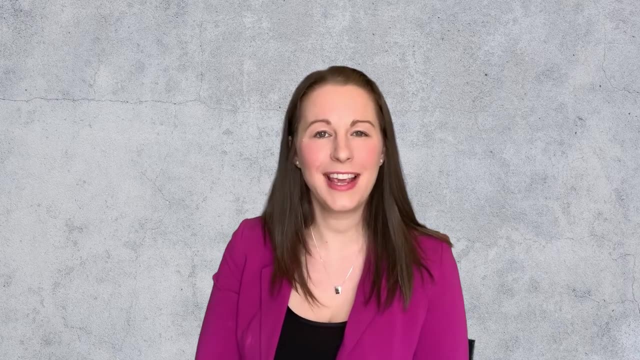 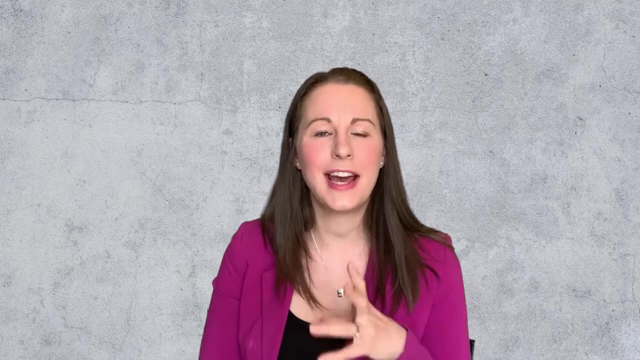 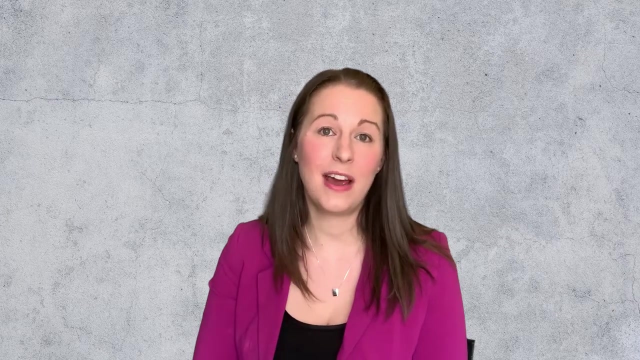 video, but just something to consider now. To just briefly touch on the inheritance tax considerations, I'd probably suggest thinking about including your children or grandchildren now, because, as a property investor, inheritance tax will definitely start to play into your life as you get older, on the basis that you have assets And when you have assets that have value. it will catch you out with the inheritance tax side of things. So by bringing in your children or your grandchildren it reduces the value of your estate now, but you still can have the benefit of those assets now as well. Now you may only want to give your children or grandchildren- 5%, 10%, and then it keeps them involved, but it doesn't dwindle away what you've already built yourself and what you want to be looking at taking. The other thing to mention is also the lending implications If you have minors, so under 18s you might. 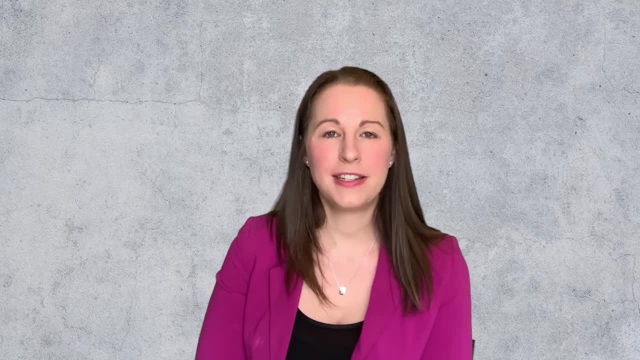 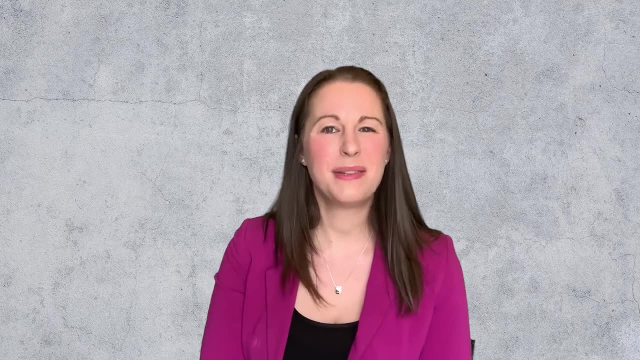 have a 15, 16-year-old child that you want to bring in as a shareholder, That's not a problem. However, you don't want to be giving them 50% of the company because the lenders may not want to lend money to you on the basis that they can't bring anything against that. 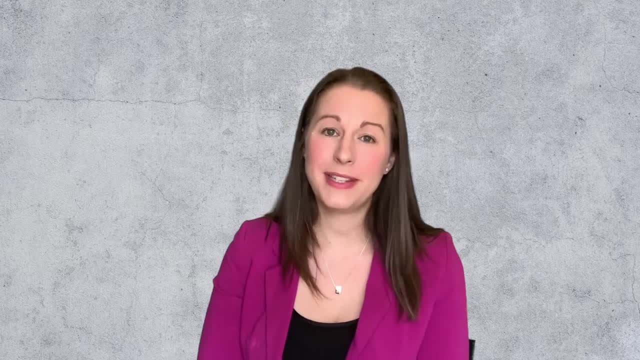 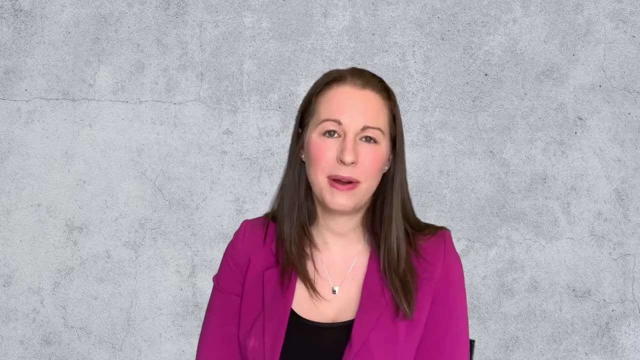 individual. Now a lot of lenders tend to look at around the 20% mark. So if you wanted to bring a child in who was maybe not 18, then you may want to have less than 20%. Also, if you're bringing other family members into the company but they're not actively involved, 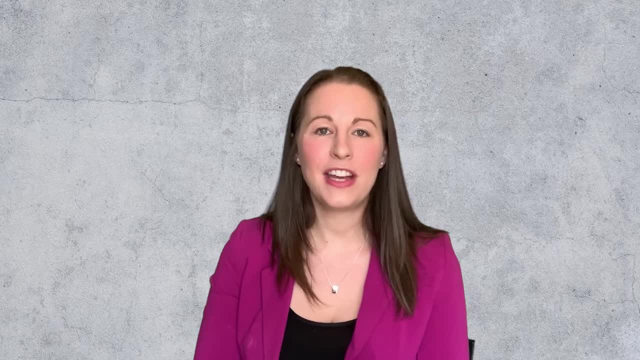 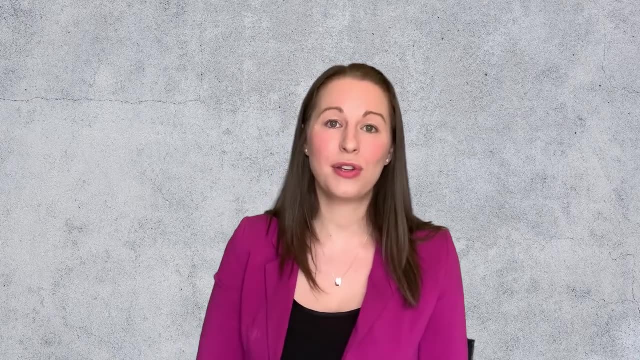 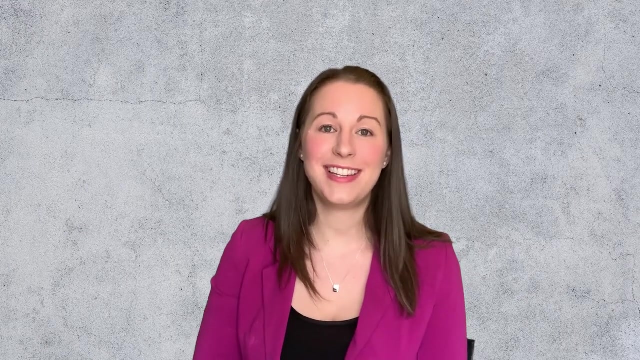 in the company, then you may need to Limit their shareholding to maybe less than 20%, because lenders tend to not look at the involvement of those under 20%. They're looking at the majority shareholders, which will still be you at this point in time to make a decision on the lending. They're likely to want personal. 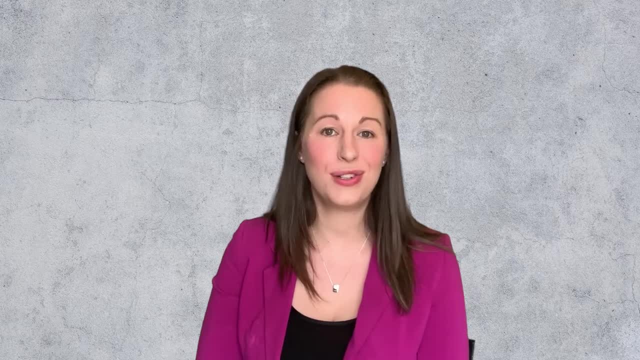 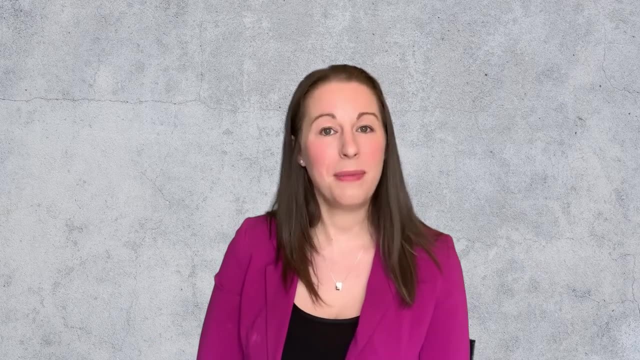 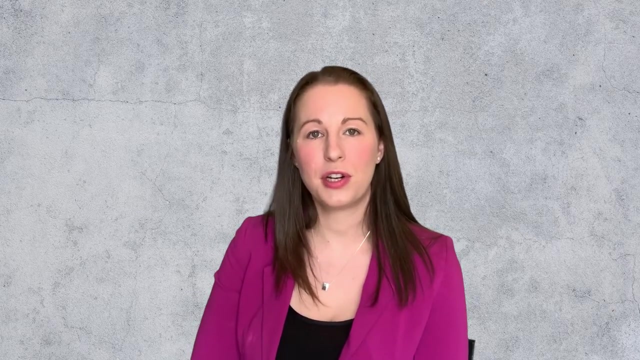 guarantees, which is kind of not a problem, as long as you're happy with that Initially. it's expected Obviously, as you build your property portfolio, you may want to start negotiating with them. One thing that you may wish to consider is setting up a group structure. Now, I'm not 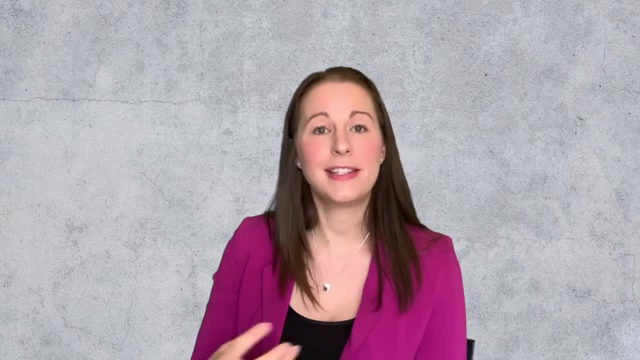 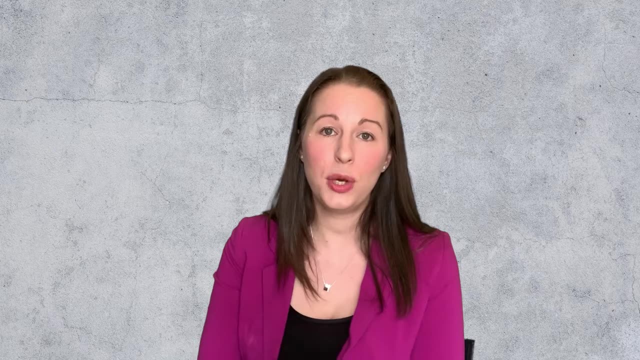 going to discuss that now. We do have a separate video on setting up your group structure, but it's something just to consider as you are setting up your property company, because it may be- rather than you as the shareholders, it may be- your holding company that wants. 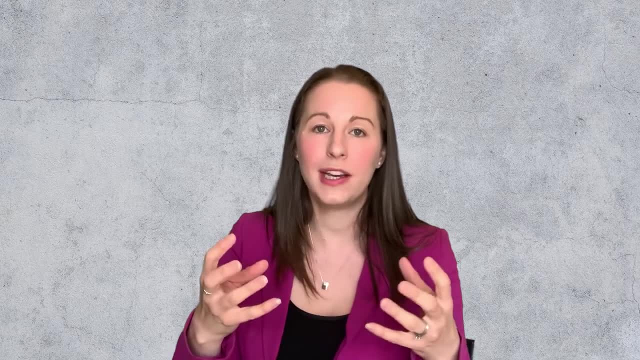 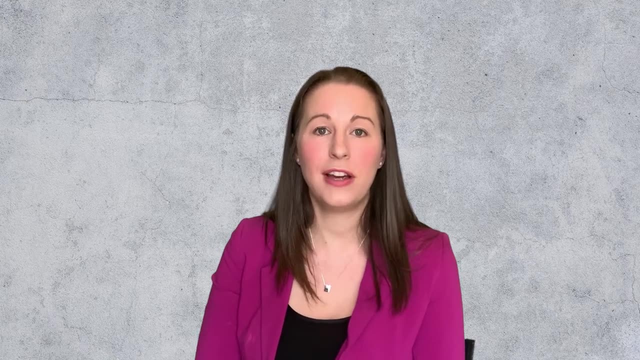 to be the shareholder and you are the shareholder of your holding company and that's where you start playing with the shareholdings with your family members. But check out the group structure video to find out how that all fits together and make it work for you and your family. 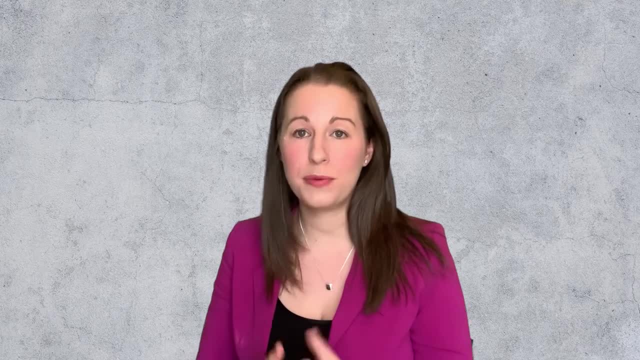 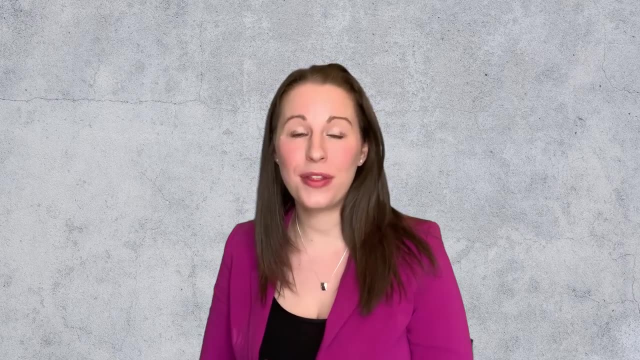 If you decide on a more complex structure and having a group structure, there may be lending implications. So I'd tend to suggest speaking to your finance broker to make sure that you've considered those options, to make sure you don't find you've got any problems. 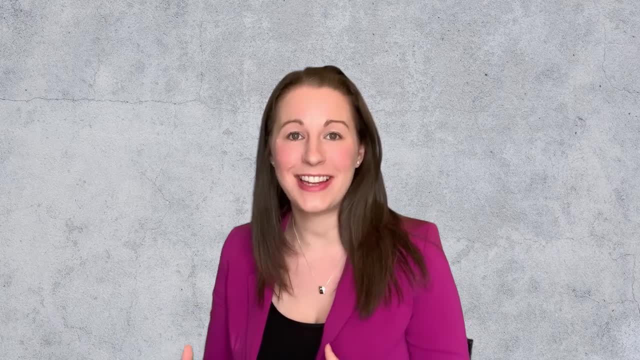 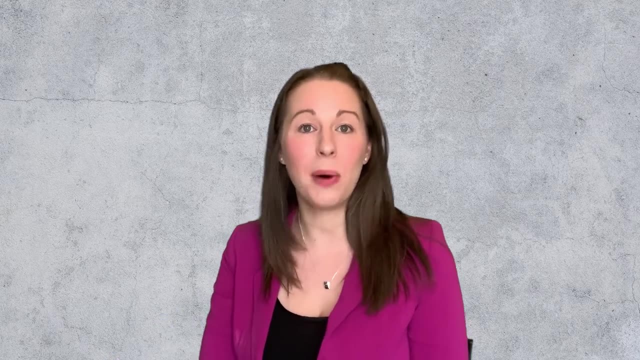 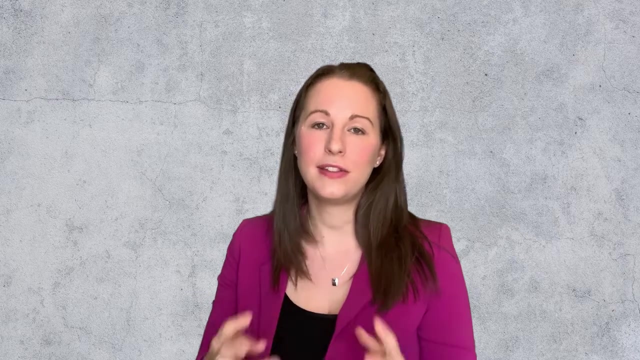 getting funding when you come to actually set everything up and get going. So that's a really bad situation to be in. We want to make sure we stop that happening. So talk to your finance broker to make sure that the structure that you are choosing to use is. going to work for you. So how do you go about setting up a property company? Well, there's a few different options. You could set up your property company yourself at Companies House. Now this costs about 10, 12 pounds at Companies House. 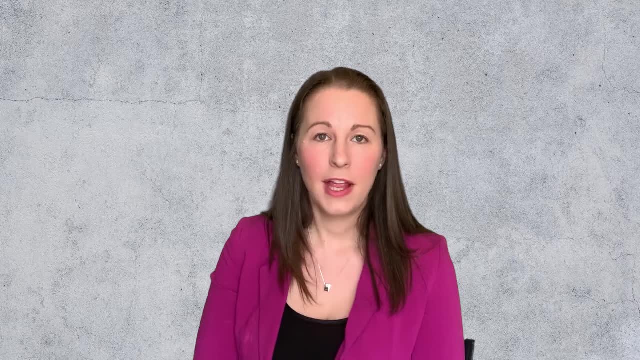 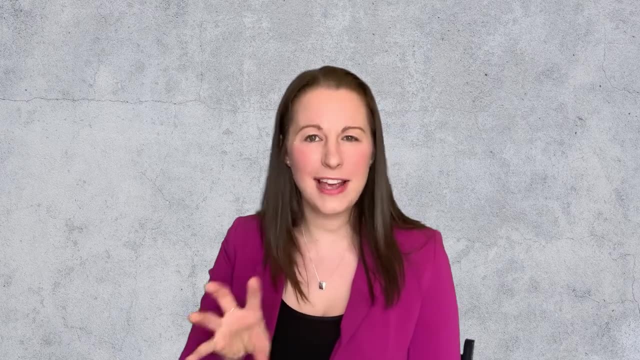 And you just go on and fill out all the information. If you're confident to do this, this is the most cost effective method of setting up your company. If you're a little less sure of how to go about setting one up, then you may want to use a company formation agent, And there's 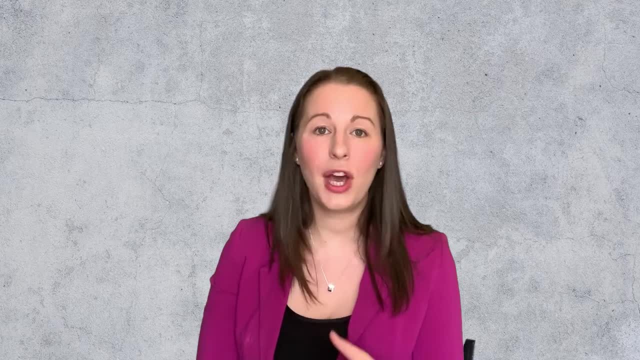 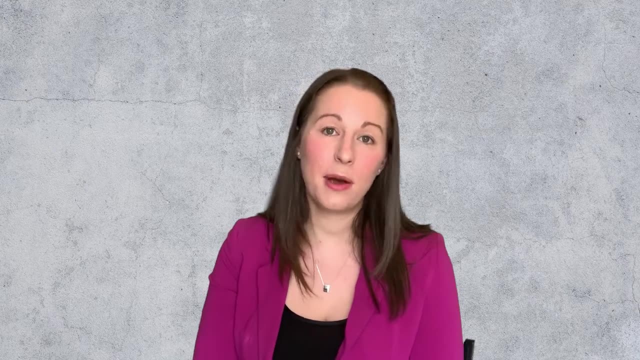 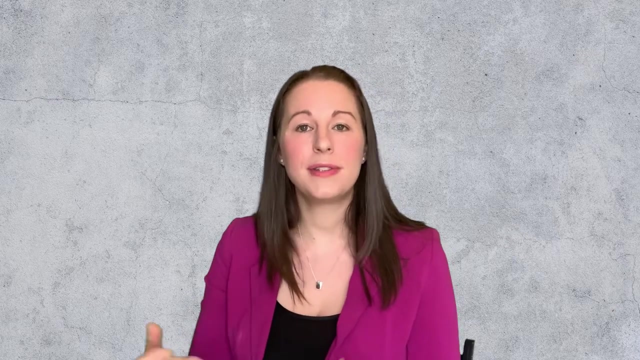 many online options available And you can go, and for a small fee you can go and fill out all the details. They'll confirm everything and get the company set up for you. Your final option is to use an accountant or a tax advisor or use a solicitor, And they'll again be able. 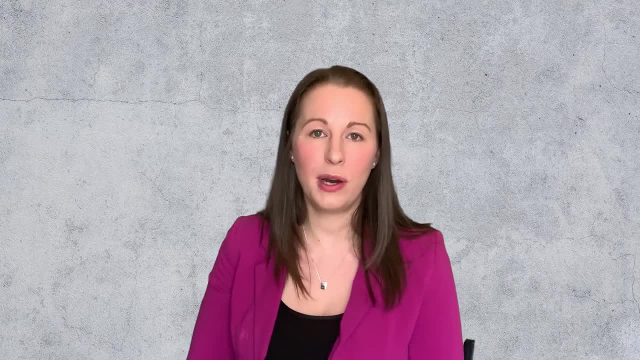 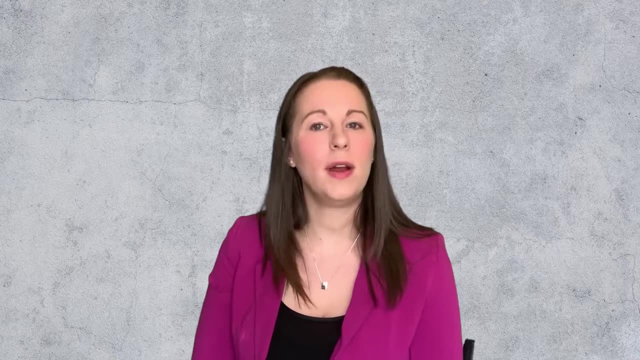 to help set it up, make sure that everything is set up in the right way. Now, in terms of what needs setting up, there's a few different pieces of paper that you will get when you form your company. One is your certificate of incorporation. So if you think, 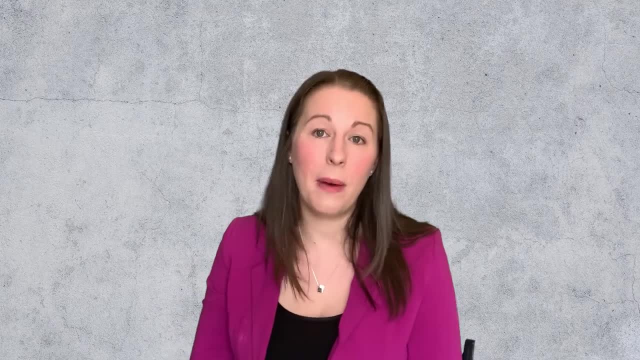 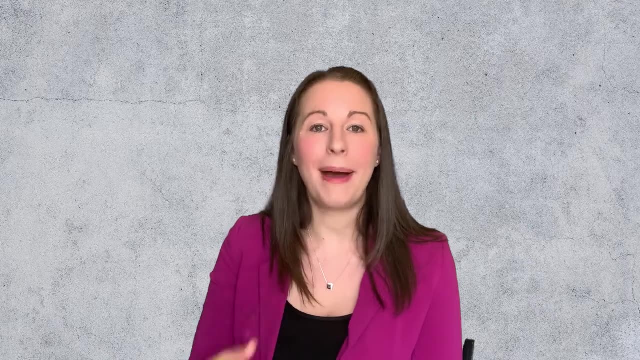 of this like a birth certificate. it's the birth certificate of the company, And it's quite a crucial piece of data, because you will need this document To be able to set up your bank account, So that's one thing that you should get when 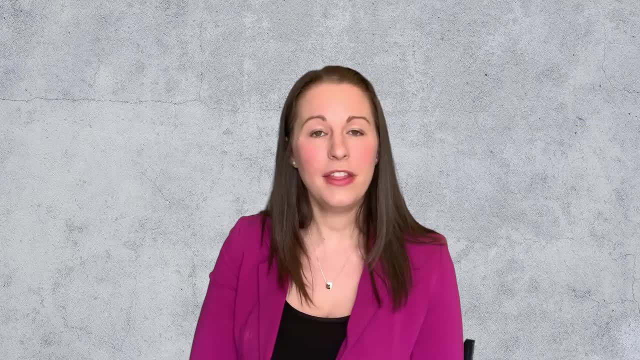 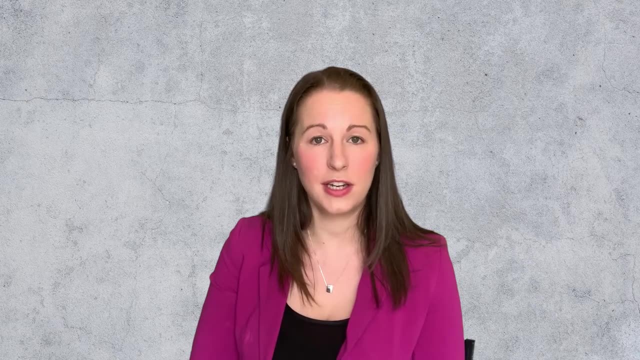 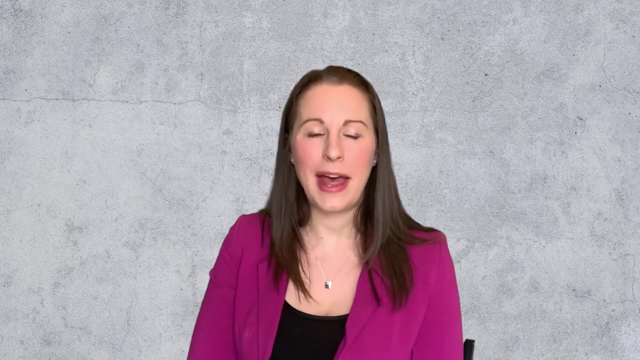 you set up your company, And that's very crucial. The other thing that you will get with your company is the memorandum of association and articles of association. Now, these documents are pretty much like the rules, rule books for your company, And they're there to help. manage if there's any discrepancies or how you are going to run your company. Now, most people will do that, But if you're going to run your company, you're going to have to make sure that you have a certificate of incorporation, So you will need to make sure that you have. 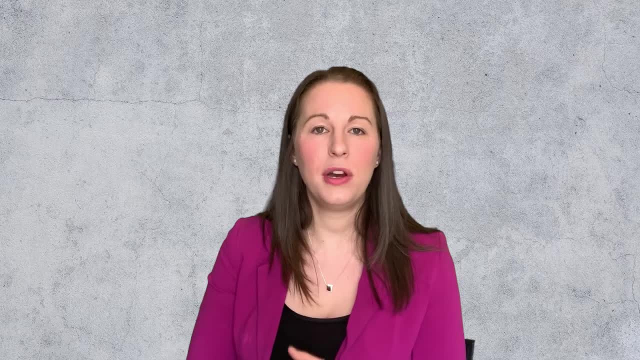 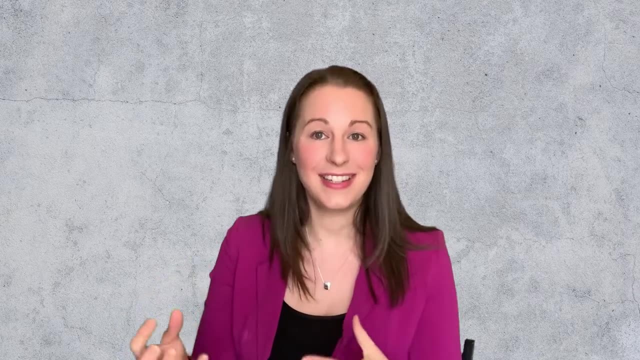 a certificate of incorporation And if you're going to run your company, you'll just use table A, which is the standard format. However, if you do want adjustments to that, then you may need to make sure you make those adjustments yourself or you may need to be using a solicitor. 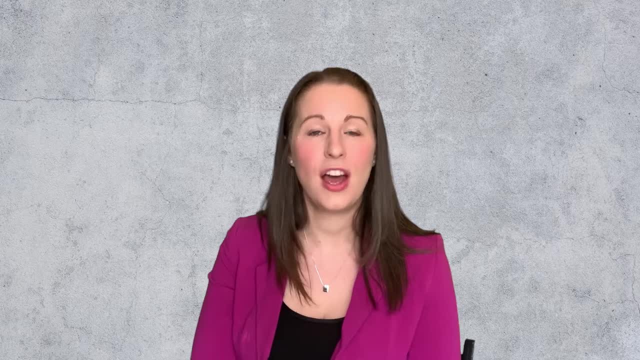 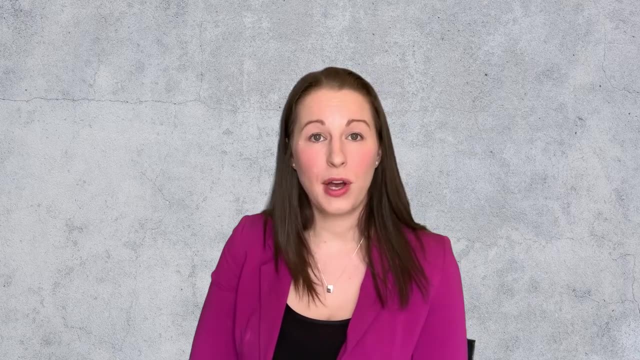 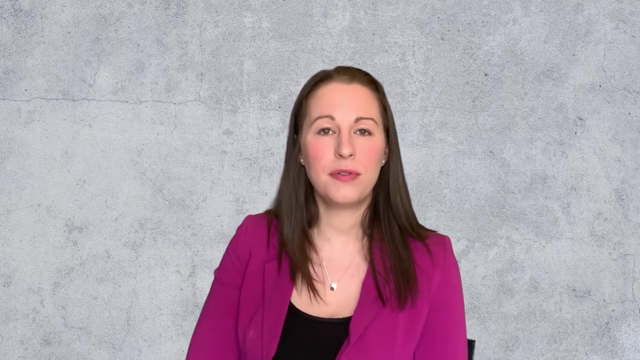 to make sure any variations you want to see in such documents are fully included. Another item you'll need to be aware of when you're setting up your company is the SIC code. So the SIC code is your standard industry classification, And these can be quite crucial. 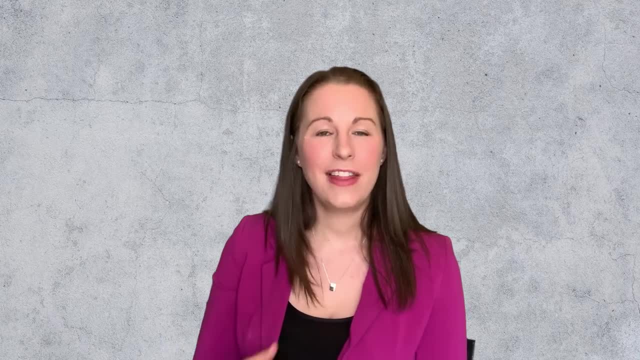 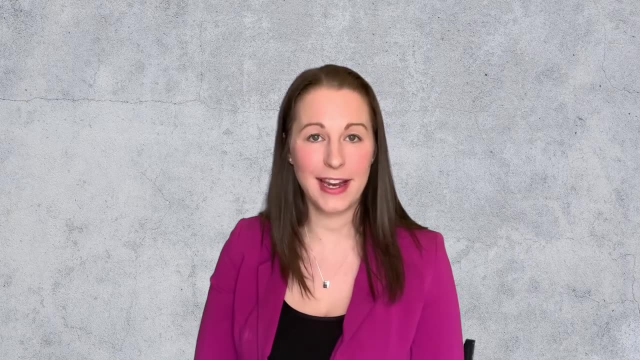 for property investors, Because if you are going for lending, the lenders will check what SIC code you have allocated to that company and will want to make sure that it's the right SIC code. So just be cautious when you're selecting and make sure you choose the right. 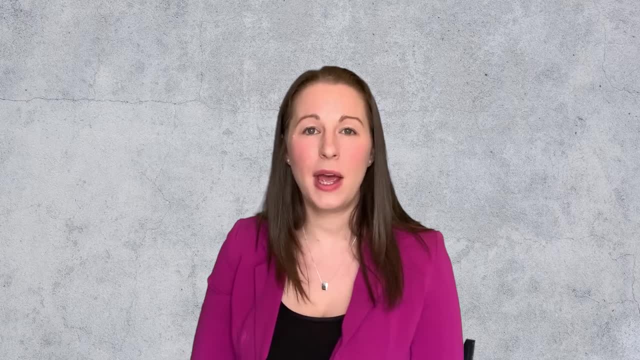 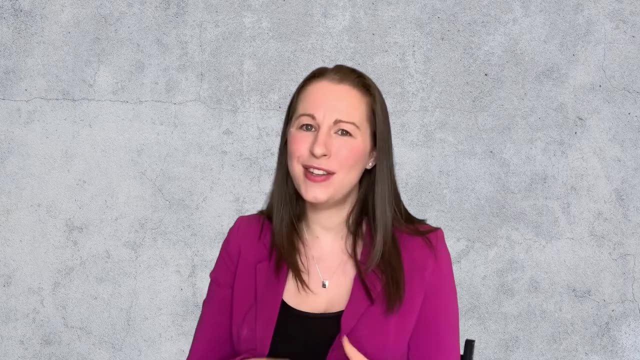 one. There's a couple of different options, but you'll tend to find other property companies, if you are aware of any, to find what the right one is. And if uncertain at all, check with your accountant and they'll be able to support you on making sure you select the 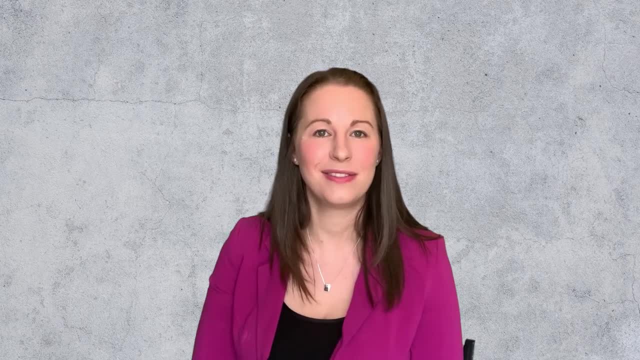 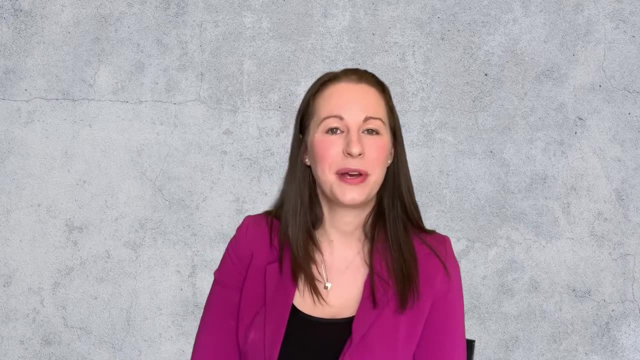 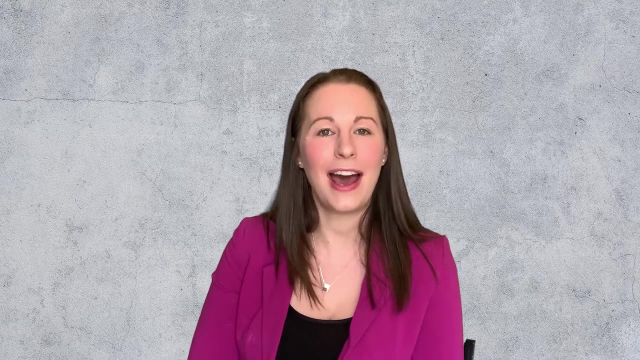 right one In terms of the timing of when you should set up your company. please check out the separate video about when to set up a company, And this will go into the different options available to you to make sure you're setting up at the right time for you and how your 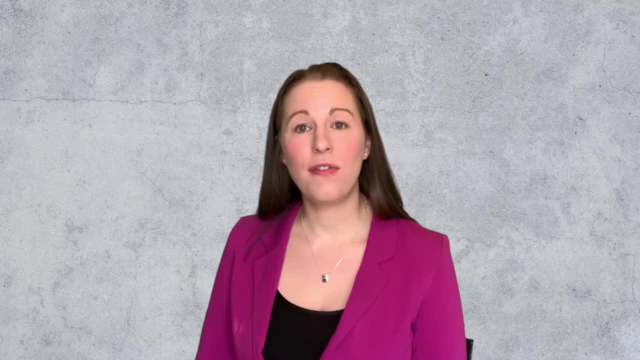 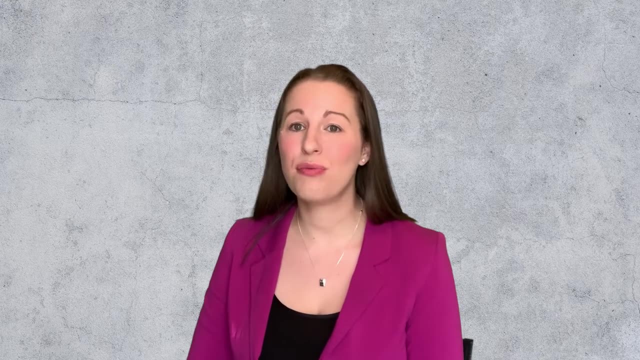 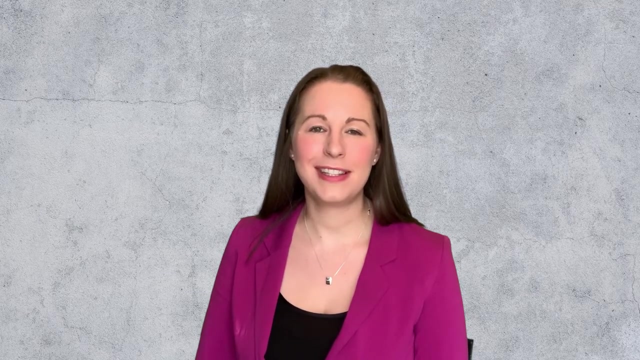 business is developing. What are the legal duties for a director of a company? Well, the legal duties are really to act with integrity, to show reasonable care and act on the right and best interests of the company. This should be relatively easy to do on the basis. it's 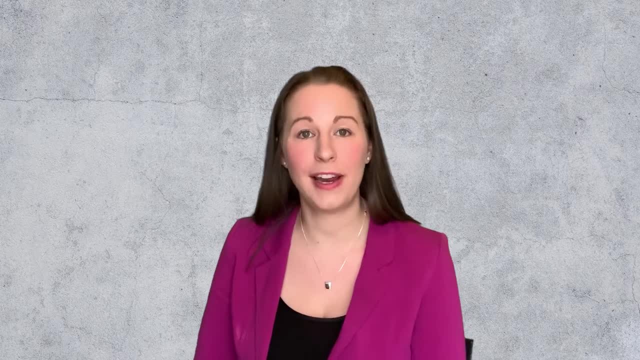 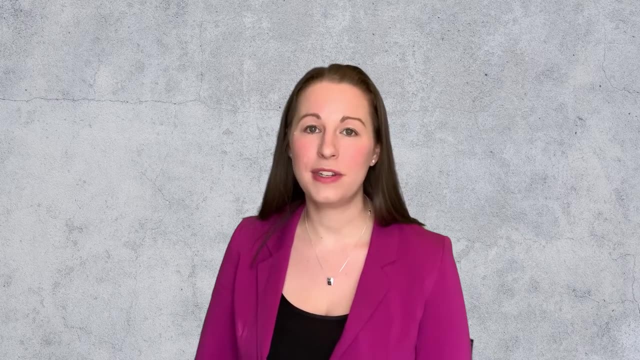 in the company's interests and your interests, which are hopefully aligned. I would recommend just making sure you read through what a director's legal duties are as you get involved in a company. They're not too long, but it just makes sure that you are fully aware of what. 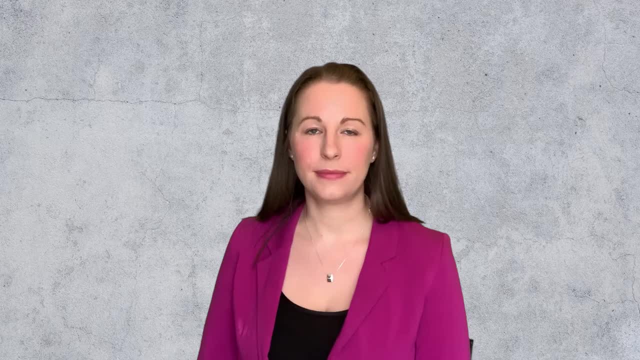 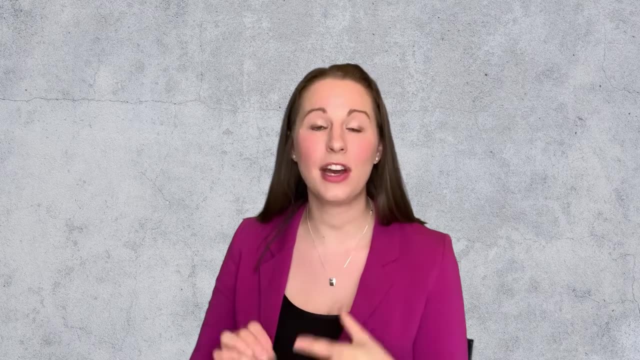 your responsibilities as you take on this role are: When you've got your company set up, you'll be be able to go and set up your company bank account and I would say you definitely need a company bank account if you're going to be trading in your company, whether that be buying to hold buying to. flip buying. to do whatever in your company, you will need a company bank account. You cannot use one of your own bank accounts for company transactions because there are tax consequences for that type of behaviour which can be quite expensive if not dealt with. Therefore, make sure. 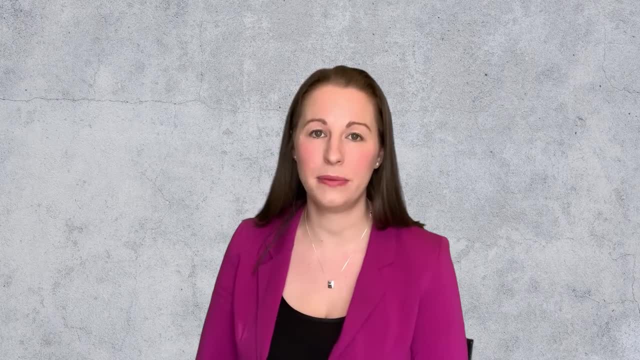 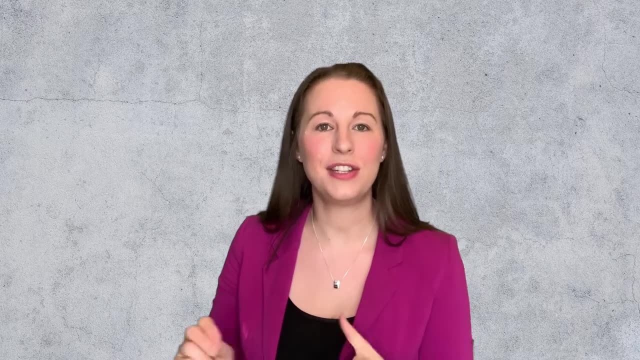 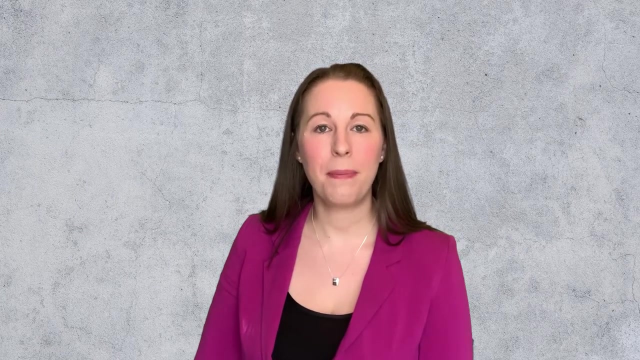 as you get trading in your company, get your company bank account set up. And finally, now that you've got your company set up, what do you need to do? What are your responsibilities As a director of the company? you will now need to prepare a set of company accounts. Now, I would tend to not. 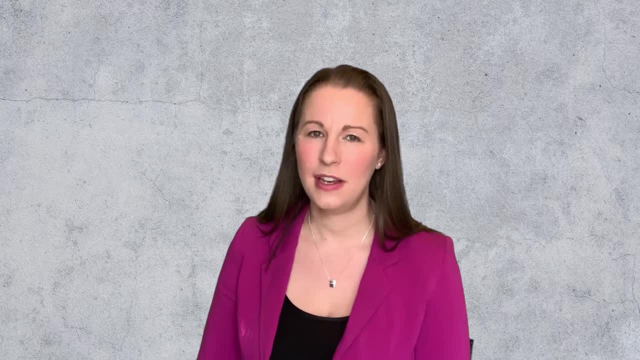 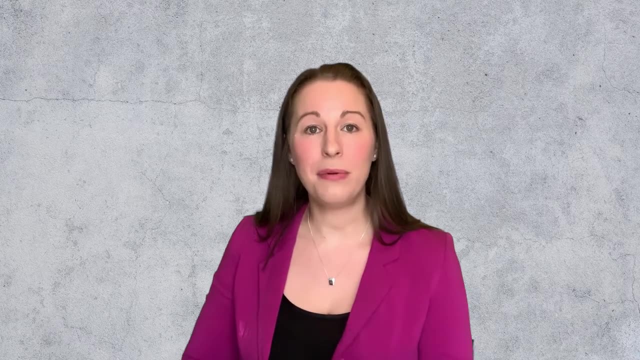 recommend you do a set of company accounts if you're going to be trading in your company, but these themselves, unless you're a trained accountant. So at that point you will need to engage a qualified accountant and in doing that they will then prepare for you a set of accounts. Now these accounts need to be completed each year after 12 months. So if you form your company in March, your year end would be the end of March. So therefore, each March is the end of your accounting period, and you will then have nine months to complete your accounting period. So that's. and that is due to be paid nine months and one day after the year end. And then you will also need to pull together a statutory set of accounts and file them with Companies House. From those accounts, you will then also look at completing your corporation tax return and collate all the tax. implications, complete the tax calculation and then submit a CT600 or corporation tax return to HM Revenue and Customs And that is due to be paid nine months and one day after the year end And the return is due 12 months after the year end. 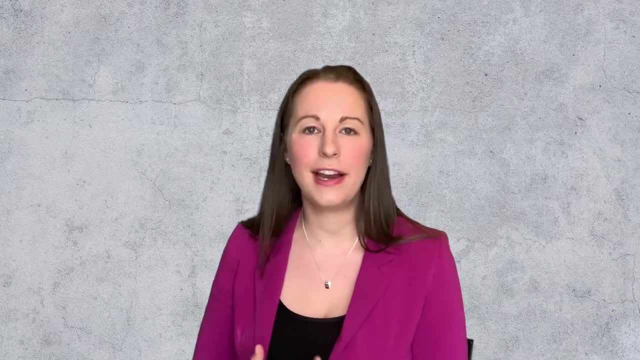 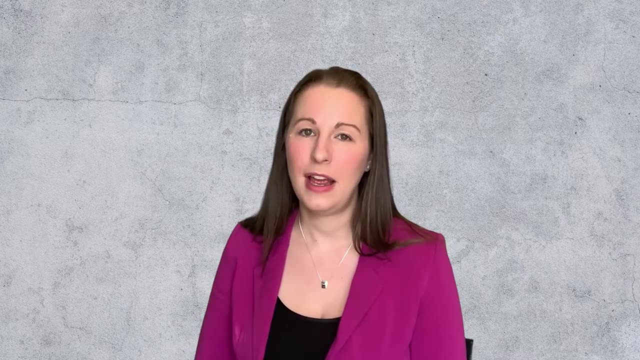 I would tend to recommend getting most of these things in as early as possible, unless there is a specific reason why you may want to leave it close to the deadline for whatever reason, And there are the odd occasion where the reason does justify leaving it right till the deadline.